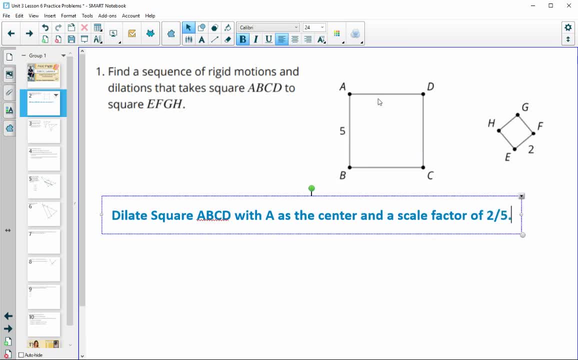 a scale factor of two fifths. so then that's going to get my square to be the same size as the other one. now I'm going to have to start bringing it over and getting it to touching the other square. so let's see, let me see if I can put this on here. so currently what I've done is just scaled it down. 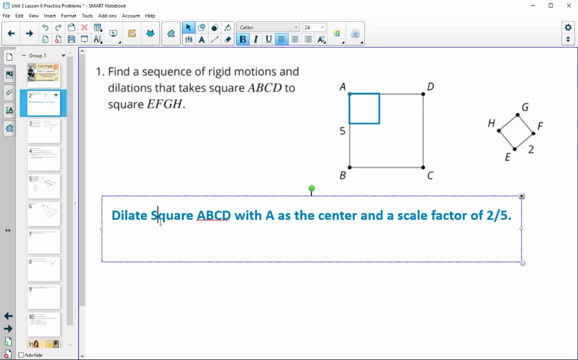 so that it's the same size. so now I'm going to get them touching by doing a translation. so I'm going to translate square ABCD by directed line segment and I'm going to take A to E, so by directed line segment, AE, which will get us here, and then I'm going to need to rotate to get it on top of the other one. 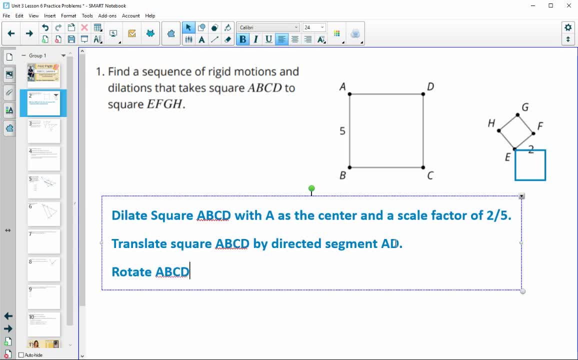 so we'll do rotate ABCD around point E, since that's what it's touching until and now. this point right here was D, so I'm going to rotate until D goes all the way over to H, so until point D coincides with point H or until D lands on. you could also change this to say: 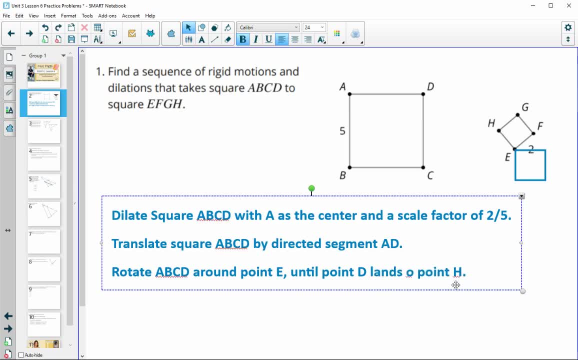 lands on point H. so either way, whichever one you like better, but then that's going to kind of bring it to the center, so that's going to get it on top of the other one. so I'm going to get it all the way like this, and then they would be, um, exactly on top of each other. 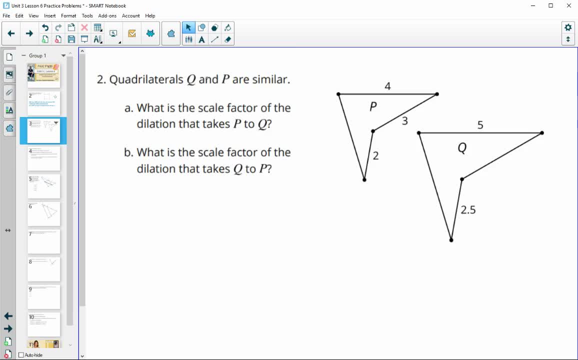 number two, quadrilateral: P, um, Q and P are similar. what's the scale factor that would take P to Q? okay, so saying that P is the original. so in this one, P is the original and you're going um to Q. so remember that you need to take a the new length. 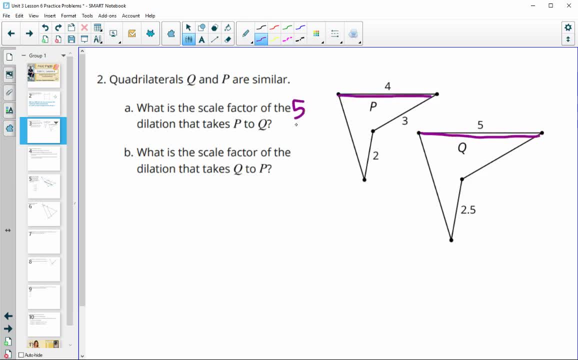 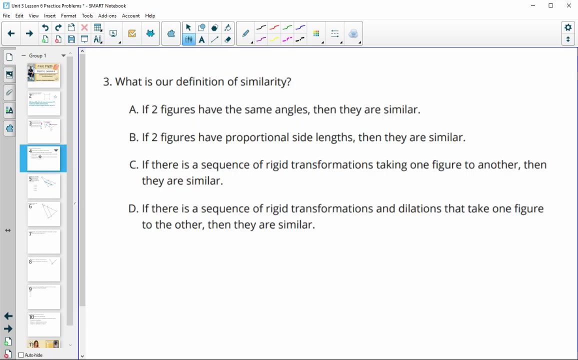 divided by an original length. so that's going to give us the scale factor taking P to Q, and then if we wanted to do the scale factor, that would take Q to P to go backwards. now our new length would be four and our original length would be five. number three: what is our definition? 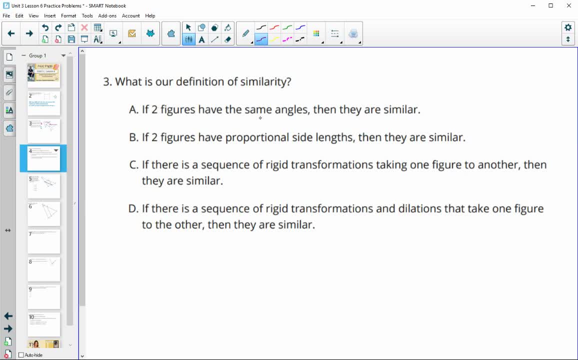 of similarity. so A just says two figures that have the same angles then they're going to be similar. that's not true. if two figures have proportional side lengths, then they're similar. that's not true. if there's a sequence of rigid transformations that takes one figure to another, then they're. 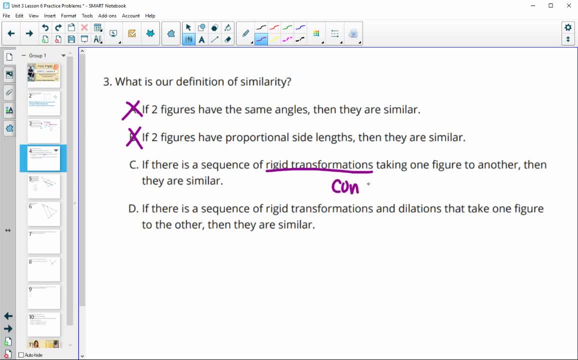 similar. if it's just rigid transformations, then they're going to be congruent. so this one's not true. so for D, now they add in rigid transformations and dilation. so the dilations is what makes them similar versus just congruent. so D would be the correct answer. 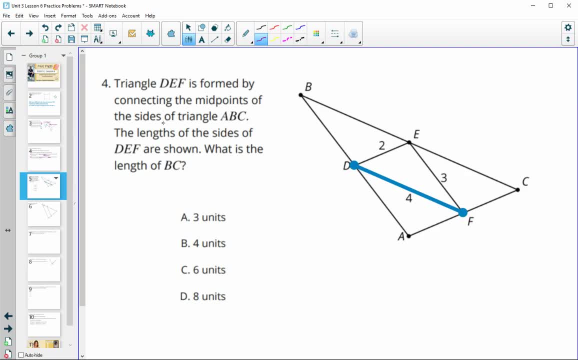 number four: triangle def is formed by connecting the midpoints of the sides of the triangle. that would mean that the lengths of um, or sorry, then the lengths of def, are shown. what is the length of BC? so now we're trying to figure out the length of this side, and so that one's going to be two times bigger than DF and 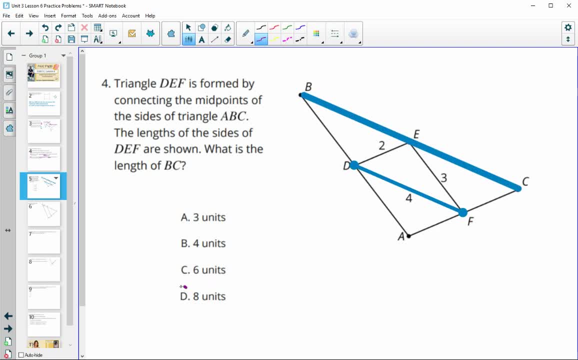 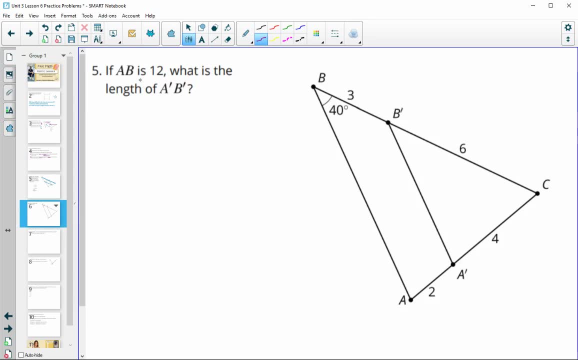 so DF is four, so BC is eight. number five, if AB is 12, okay, so we've got um, this segment right here is 12.. then what is the length of A Prime, B, Prime? so we're trying to figure out this one. so we need the scale factor to help us with this one. um, and sometimes this scale factor can be kind. 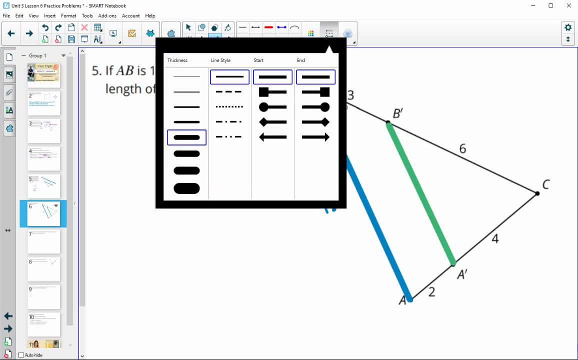 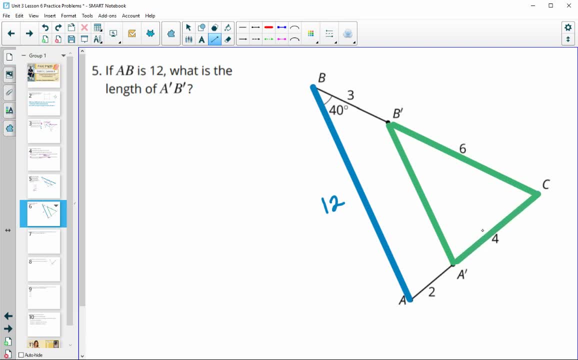 of confusing. so let's take a look at um the triangles being formed here. so we've got this top triangle here and um new length for BC. if we're looking at it is six And the original length for BC, okay, was this whole length here of nine. So when we're trying to come up with the scale factor, 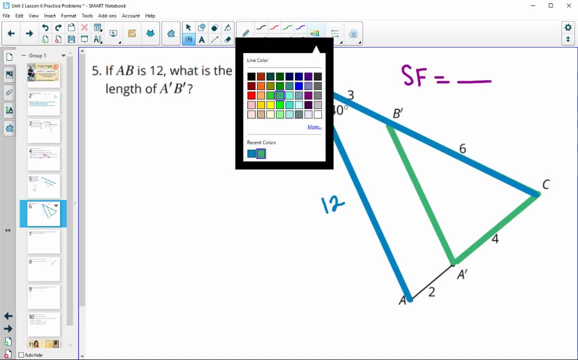 remember we do the new length and the new length B prime, C prime is six and the original length was nine, So the scale factor in this case simplifies down to two-thirds. And so then, if we're trying to figure out this one, going from AB to A prime, B prime. 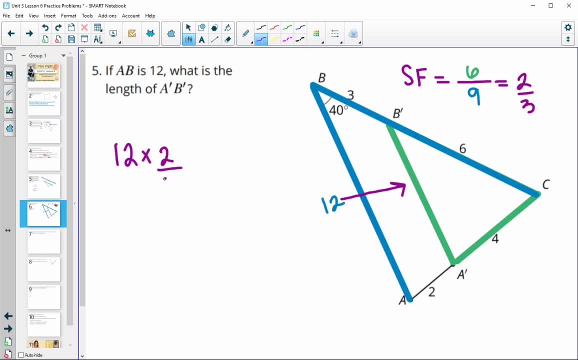 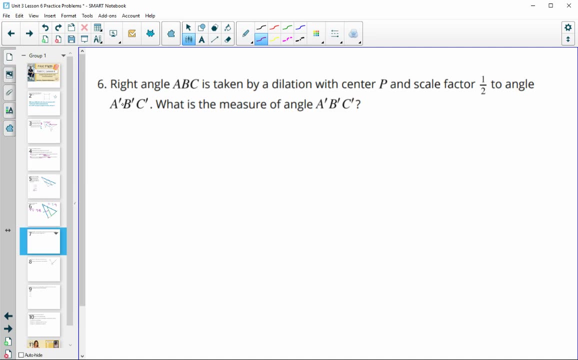 then we would take 12 times the scale factor of two-thirds, And so that would give us 24 over three or eight for the length of A. prime B: prime Number six says that right angle ABC is taken by a dilation with a center of P. 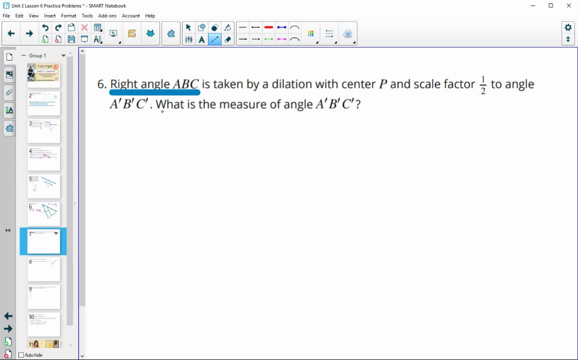 and a scale factor of one-half to angle: A prime, B prime, C prime. What's the measure of A prime, B prime, C prime. So remember, dilations do not change angle size. So since it started as a right angle, it's going to stay as a right angle that has a measure of 90 degrees. 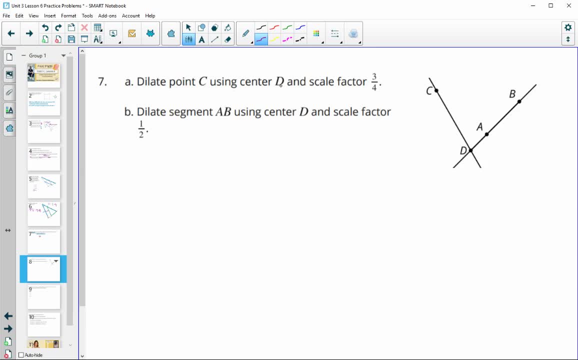 Number seven dilate point C using center D and a scale factor of three-fourths. So when you're doing this you need to have a ruler so that you can measure how far the point is from the center. So I'm going to get my ruler here and then we'll be able to measure how far point C is from D. And this will be different on your scale. So I'm going to get my ruler here and then we'll be able to measure how far point C is from D, And this will be different on your scale. So I'm going to get my ruler here and then we'll be able to measure how far point C is from D. And this will be different on your scale. So I'm going to get my ruler here and then we'll be able to measure how far point C is from D, And this will be different on your scale. So I'm going to get my ruler here and then we'll be able to measure how far point C is from D. And this will be different on your scale. So I'm going to get my ruler here and then we'll be able to measure how far point C is from D, And this will be different on your scale. So I'm going to get my ruler here and then we'll be able to measure how far point C is from D. 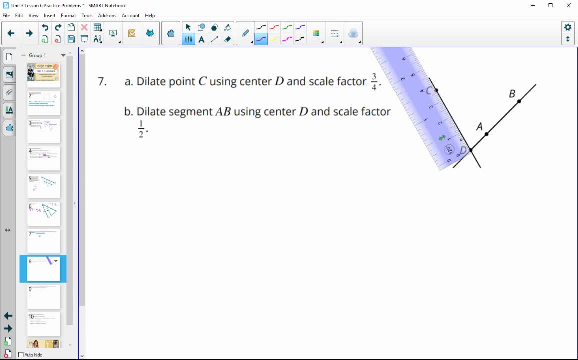 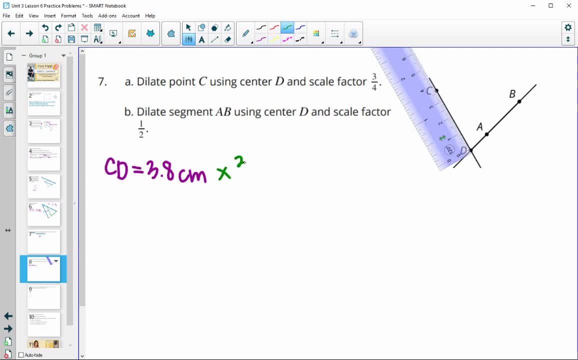 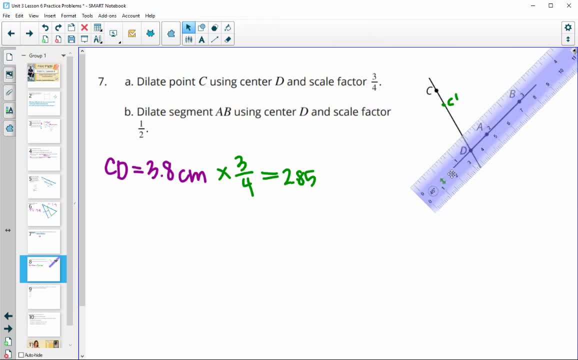 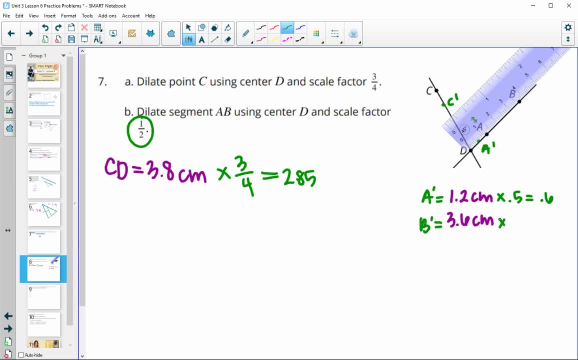 And then B prime, we're going to take 3.6 and multiply that by a half, and so that's going to be at about 1.8 centimeters, And so that's going to be at about 1.8 centimeters. 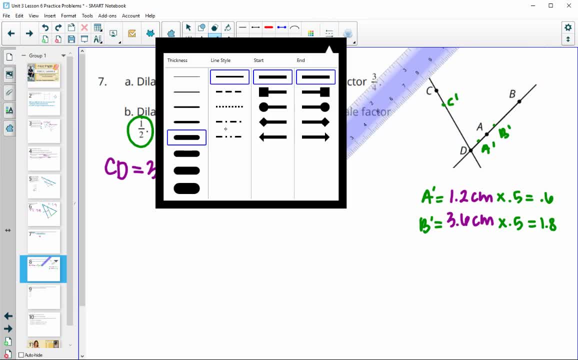 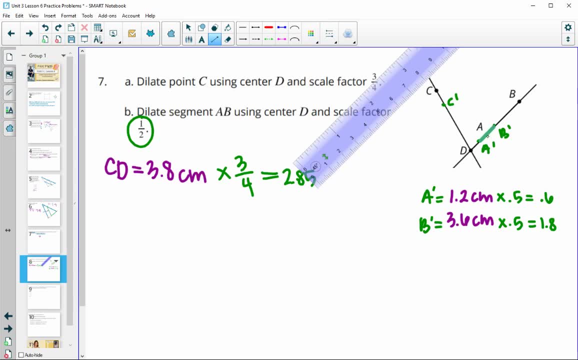 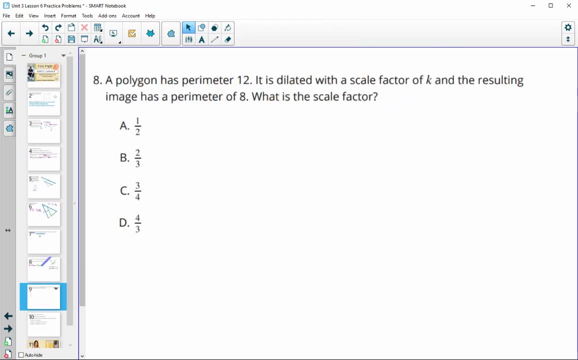 So not only do the points move closer to D from that dilation, but the segment also gets half the length of the original Number A, 8,. a polygon has a perimeter of 12 and it's dilated by a scale factor of K and the resulting 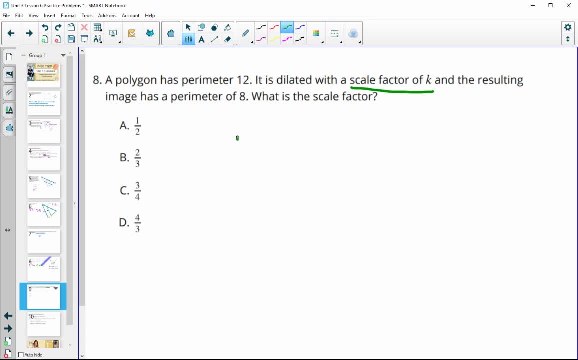 image has a perimeter of 8.. So what's the scale factor? So remember, for scale factor you do new measurement divided by original. So our new perimeter is 8, our original perimeter was 12, and then we can simplify those by dividing by 4.. So 8 divided by 4 is 2, 12 divided by 4 is 3,.